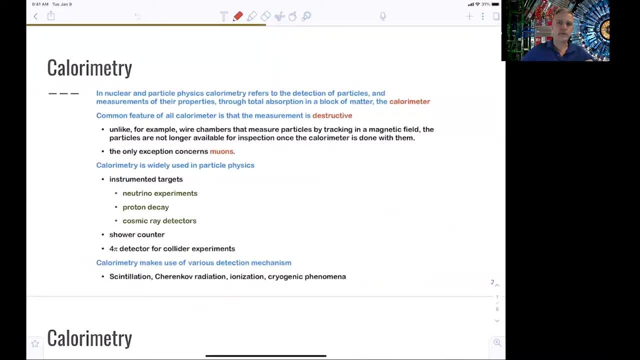 we try to destroy them. The exception to this might be a muon which might, at high energies, deposit only a small fraction of its energy in the colorimeter, or a neutrino which just flies through without having any interaction. But the purpose is really to measure energies by destroying the particle, And it's widely. 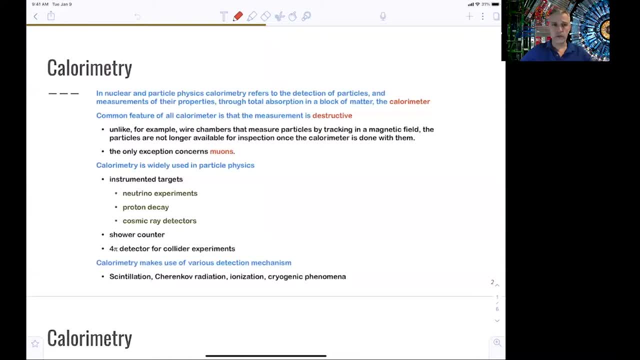 used in all kinds of areas of particle and nuclear physics: Neutrino experiments, proton decay experiments, cosmic ray detectors, collider experiments and so on. And in collider experiments specifically, the idea is to build the detector such that it completely surrounds the interaction. 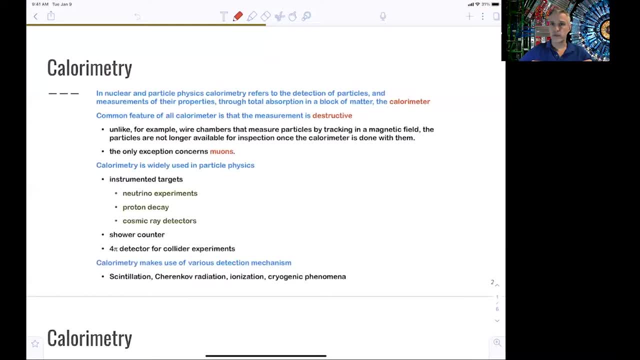 region such that you don't lose energy from the collision just passing through an uninstrumented area. The detection mechanism can vary quite a bit. We use scintillators a lot. We use silicon in some modern detectors, We use this ionization. We use Cherenkov detection. We use sometimes 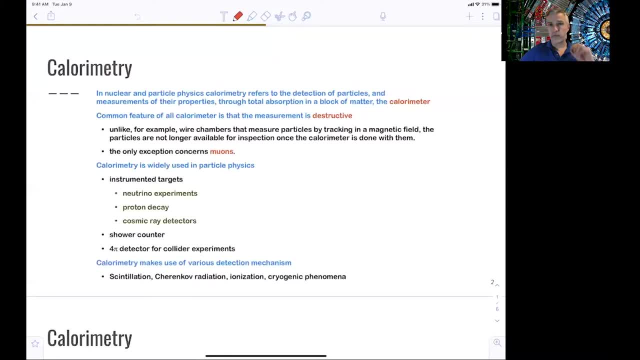 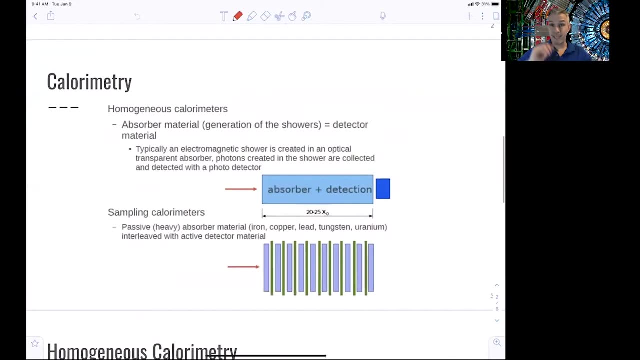 cryogenic detectors which are very sensitive to very small energy depositions, And they can be quite useful. They are used in dark matter experiments or in neutrino-less double beta decay experiments, for example. Again, conceptually you can differentiate between homogeneous colorimeters and sampling. 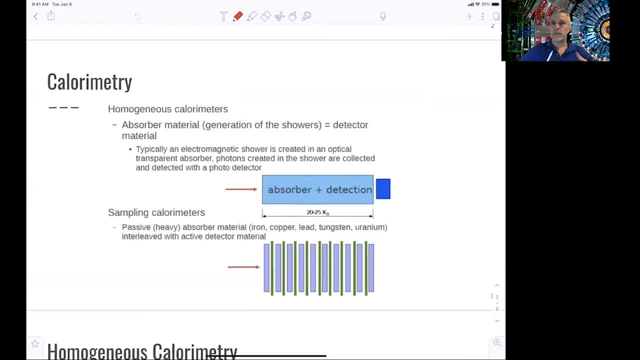 colorimeters, The homogeneous colorimeters. basically the entire absorber material is equal or is the same as the detector material. So an example for this is lead glass, which is often used. So what you do then in the colorimeter if you induce electromagnetic and nuclear showers? 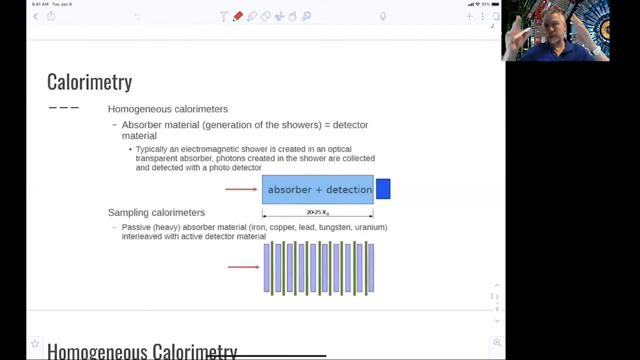 you can use the light from a light source. and you can use the light from a light source And then the energy of the incoming particle is converted into photons, And then what you need is a photodetector which then measures the number of photons coming out of your detector. 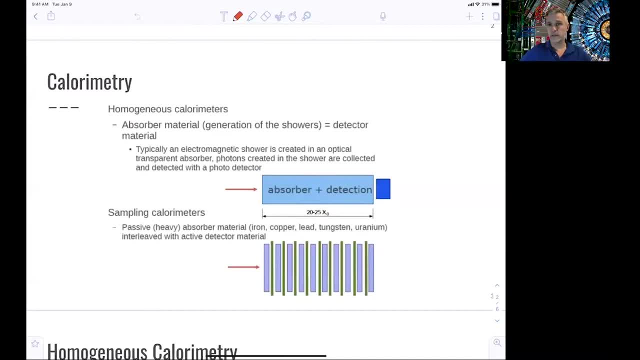 material. For this to work, the detector needs to be transparent. Alternatively, one can use sampling experiments: sampling detectors, where you have the heavy material being used in order to induce a shower and then the detection material in order to induce a shower. 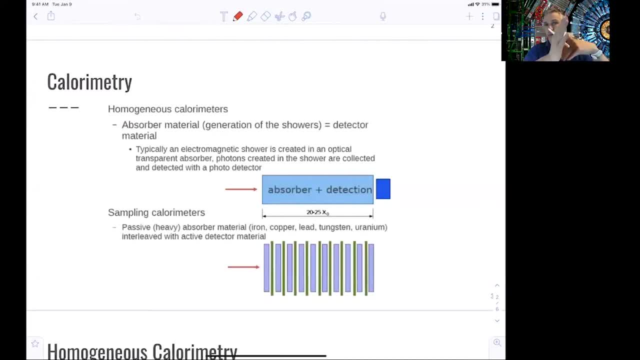 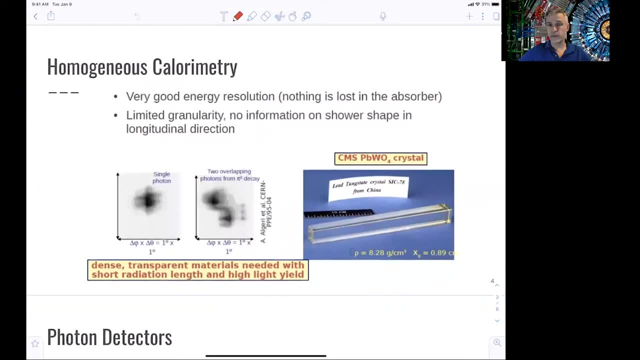 And then you have a lot of energy coming out of your detector material And that's why this is so important. So the energy of the incoming particle is converted into photons And then to count again the number of photons. So homogeneous calorimeter have typically very good energy. 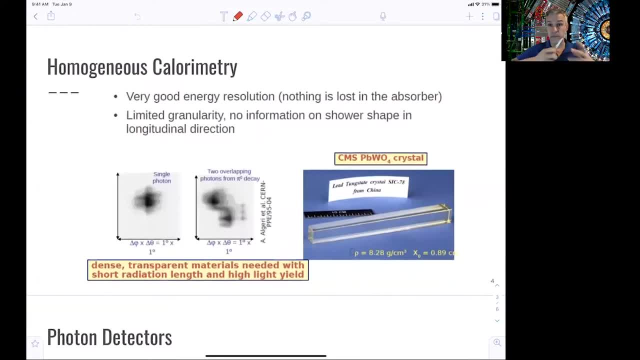 resolution, And the reason for this is that nothing gets lost. Everything is being measured in the absorber, which is the detector, But that leads into some limitations, For example that the granularity of the detector is typically limited, And then there's no longitudinal information. 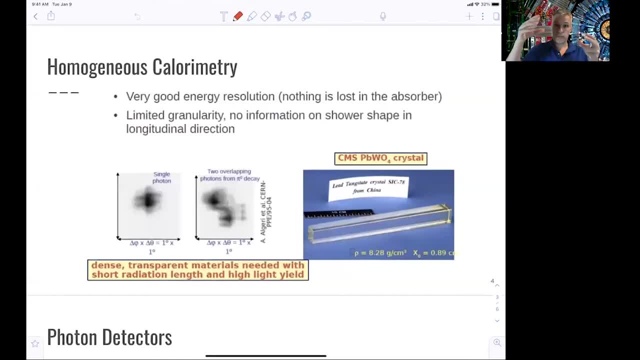 about the shower development. You basically have one block, for example, a lab block which is shown here, the tungsten block which is shown here, used for the measurement Right. so you produce photons, And so then the photons need to be measured. 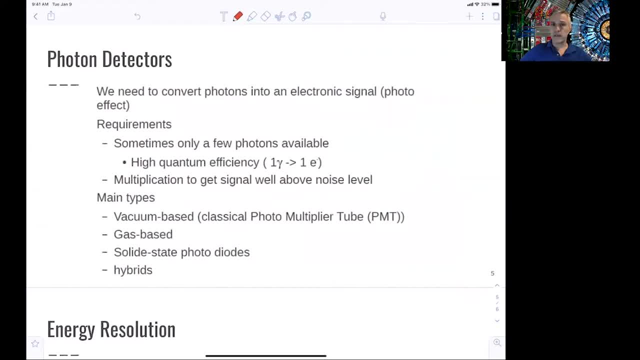 And then it's done with photodetectors. Here the range of requirements is quite big. Sometimes you want to be able to measure every single photon, So the quantum efficiency needs to be quite high. In other detectors you need to be. 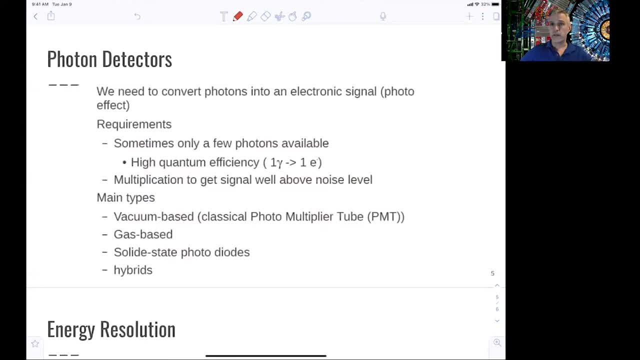 able to put this detector in a radiation-hard environment And so that then changes. The main types available are the old-fashioned photomultiplier tubes, which actually become quite sophisticated PMTs. There's gas-based photodetectors, There's solid-state detectors, which are quite popular. 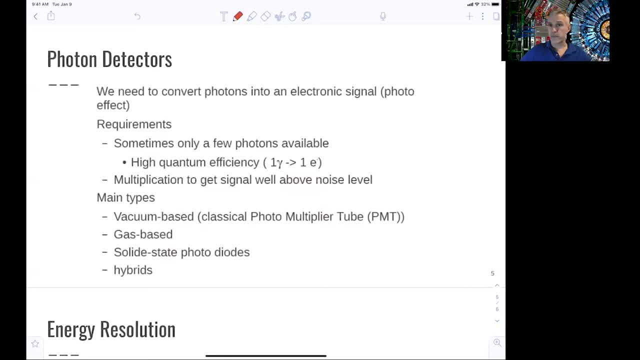 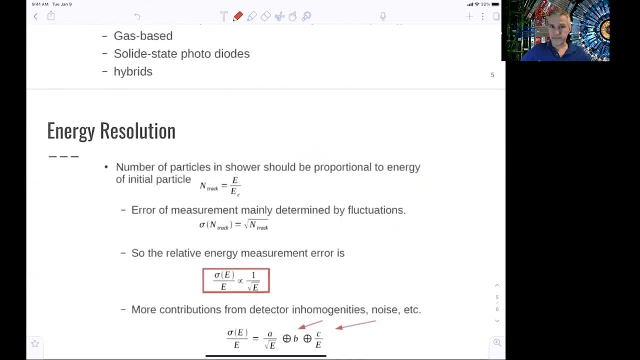 so-called SIPM, silicon photodetectors, or some hybrid modules of those. So the energy resolution in a calorimeter depends on a number of things. As I was saying, one measures the number of particles being produced in a shower, And so that's just a counting experiment. 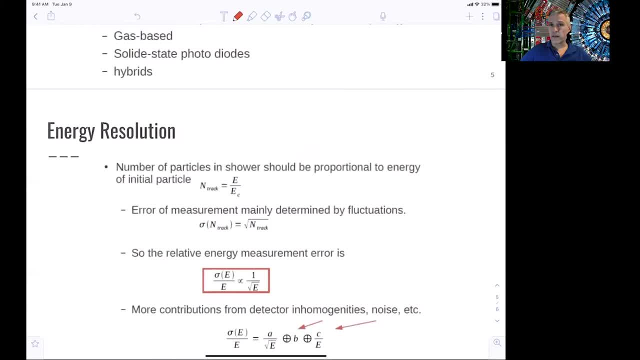 And the uncertainty of that scales with the square root of the number of particles produced or measured, And so here we have a square root n term. So the relative energy measurement has an error which is 1 over square root of the energy. 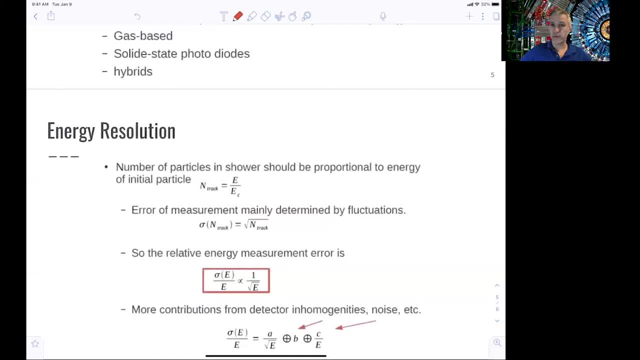 And then there's more contributions. There's constant terms which come from inhomogeneity: Right, Right, Right, Right, Those are elements where there's just no detector, no equipment in the direction of the particles. Those can be overlap regions or regions.